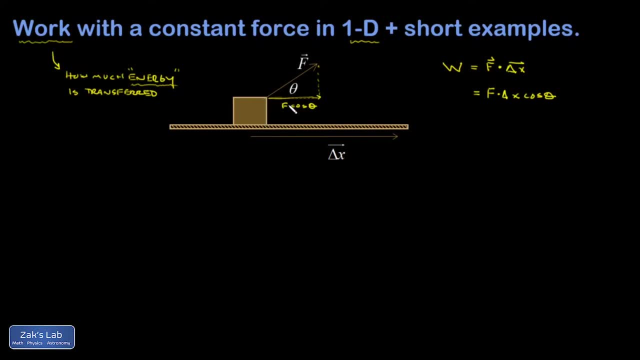 is really constrained to this surface. then there are other forces cancelling out the vertical component and that does just doesn't matter for increasing the energy of the block. all right, so there's our basic definition, and i want to look at the units of work again. a notation for that is to put it in brackets, and if i have force here, 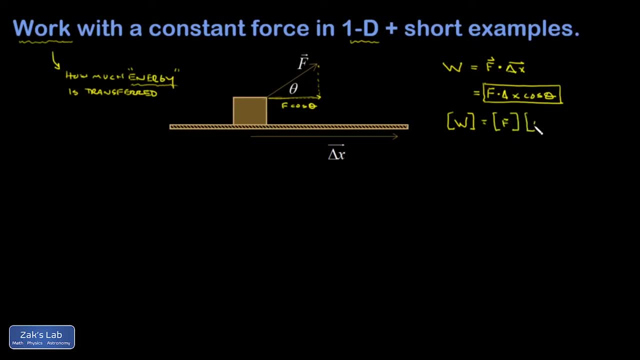 and displacement after that, and then the cosine is unitless. i don't have to worry about that piece. then the units of work must be newtons multiplied by meters, and there is a special name for this and it's called joules, and you may already be familiar with this. but joules are a unit of energy, which is no surprise. 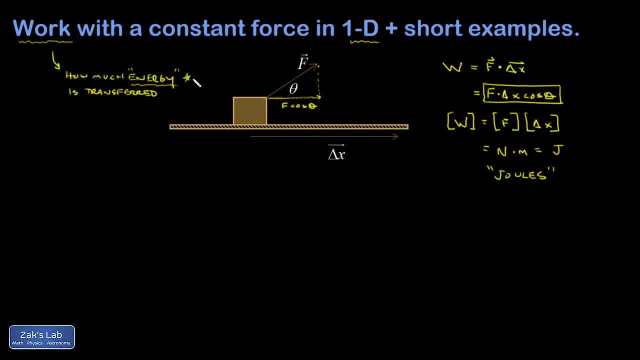 given what we're trying to do here. we're trying to calculate how much energy is transferred. so i want to do two very simple examples. first, let's suppose that the force is 100 newtons. i don't even know what the mass is, but i'm assuming. 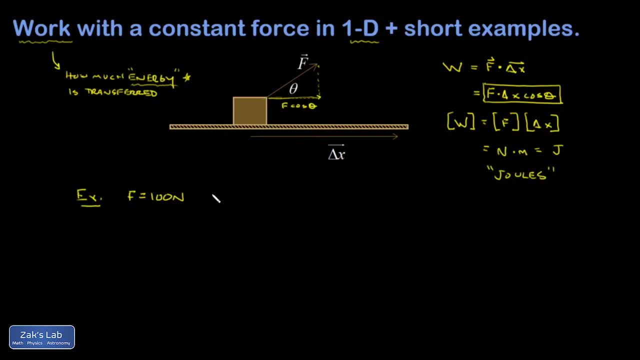 here that it's heavy enough to not come off the ground with 100 newton force. i'm going to put an angle of 35 degrees in and i'm going to put a delta x of 10 meters. in other words, we use a 100 newton force angled at 35 degrees above the horizontal. 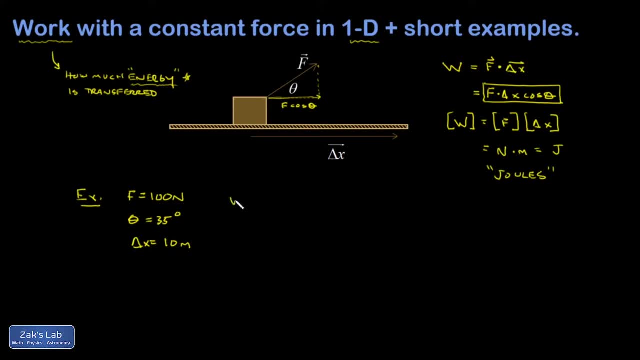 to drag a block by 10 meters and i want to know how much work is done during that process. i'm going to go ahead and work down here. so it would be an f, delta, x, cosine, theta, where theta is the angle between the force vector and the displacement. 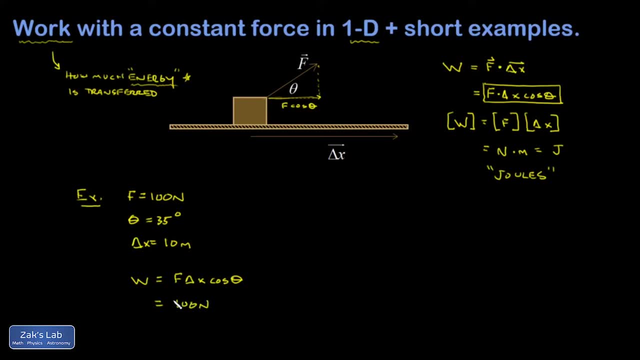 vector and i get 100 newtons multiplied by that 10 meter displacement cosine, 35 degrees, and i'll find out how much energy was pumped into the block during this process. i get 819 joules if i just keep three sig figs. so 819 joules okay. in the second short example,